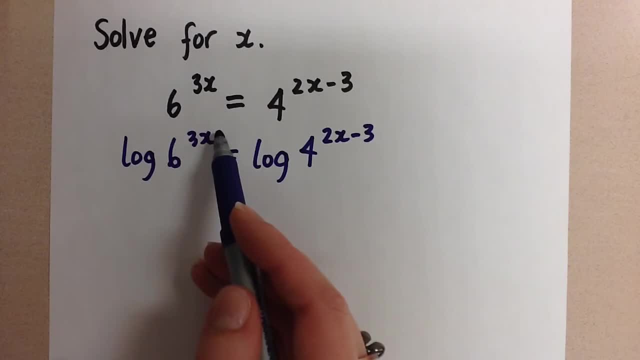 the log. here we can remove the exponent using the power law from our laws of logarithms and bring it out to be a coefficient. And the same thing with this exponent here. it can be a coefficient here, And so this works to get rid of the exponents. and now we have 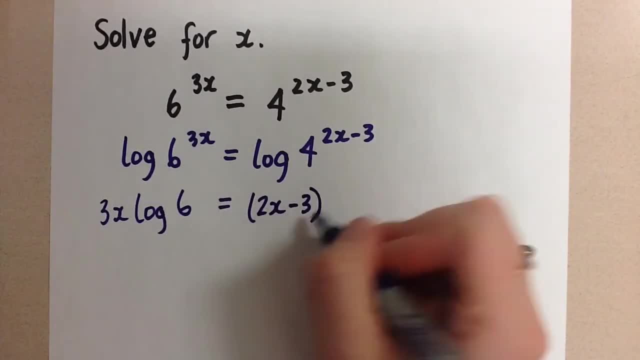 let's do like this: Now we have the variable x down into the equation and we're going to be able to solve for it. So I have an x on this side and I have an x here. I'm just going to distribute. 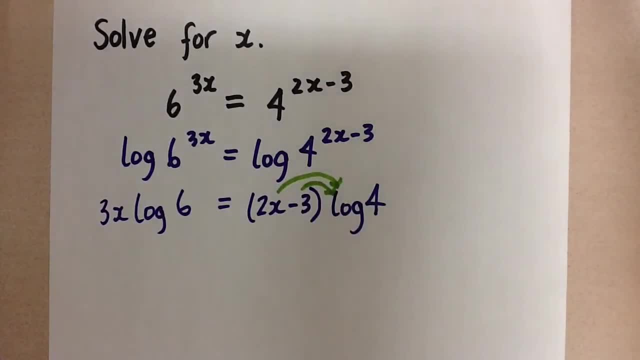 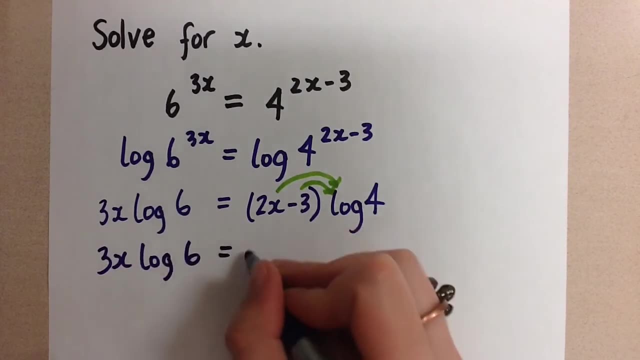 and multiply the two terms in the brackets with that log 4. to simplify Our next line: 3x log 6 equals 2x log 6.. 4 minus 3 log 4.. You can see that we have an x term here and an x term here, So we have to get these. 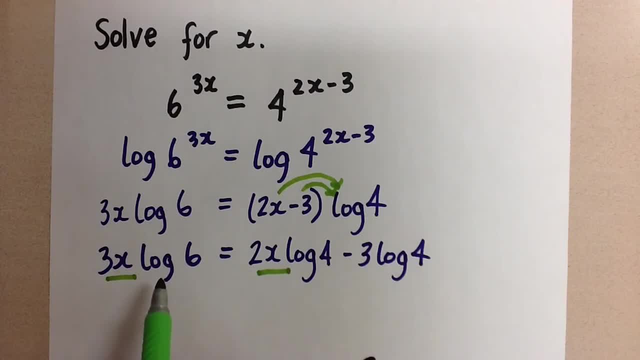 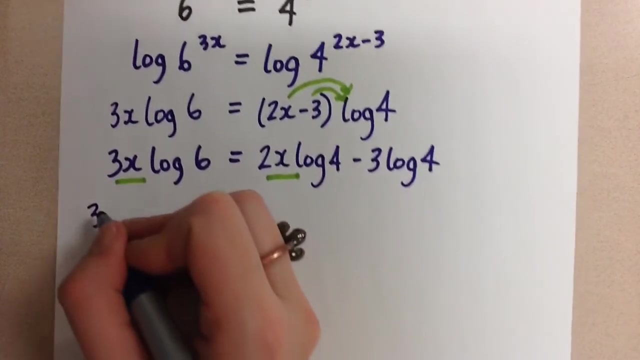 two terms on the same side so we can solve for that x variable And then we'll keep this constant here, this number minus 3, log 4, on the right-hand side. I'm going to bring over the. let's bring this up. 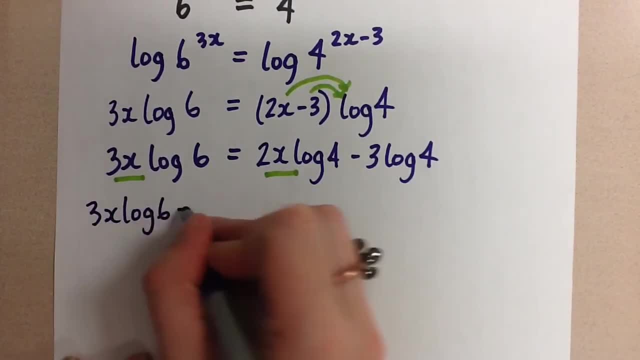 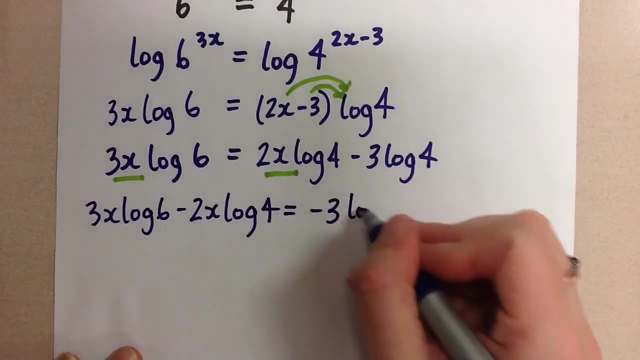 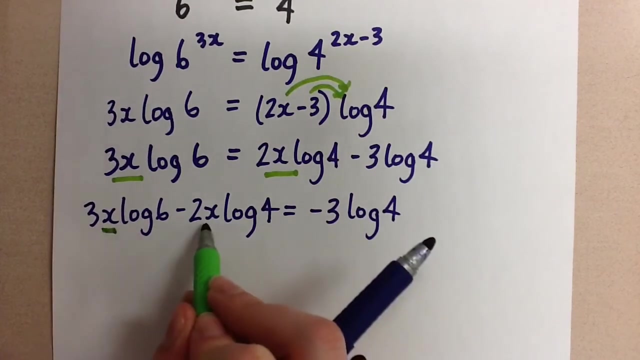 I'm going to bring over that 2x log 4 by subtracting it And we have negative 3 log 4 left on the right-hand side. We want to get that x by itself. So we have this common x factor in both of these. 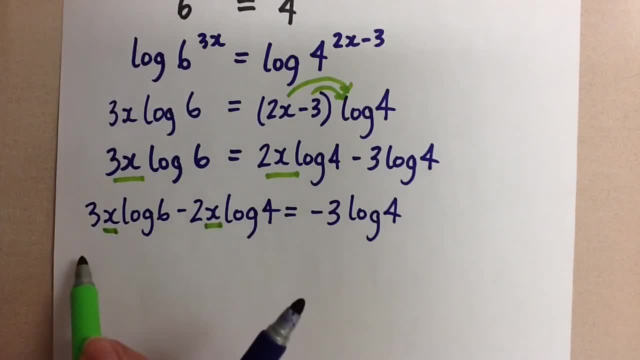 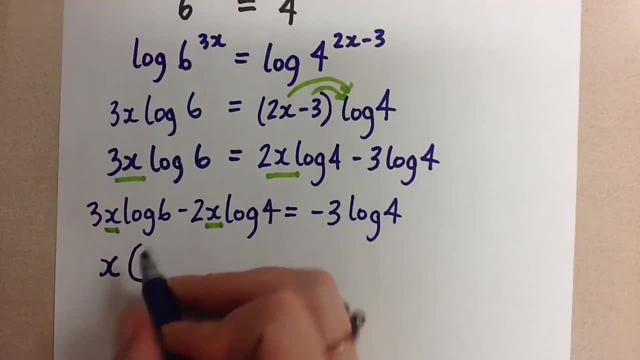 terms. We can pull out the x to the front and factor it out, And so that way we have this ovary. This looks like this: Bring the x out From this term, we're left with 3 log 6.. And in this term, 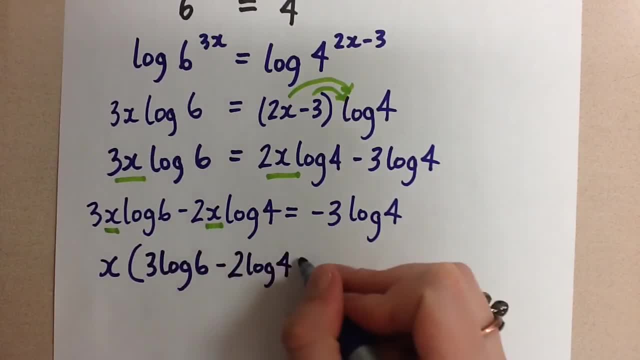 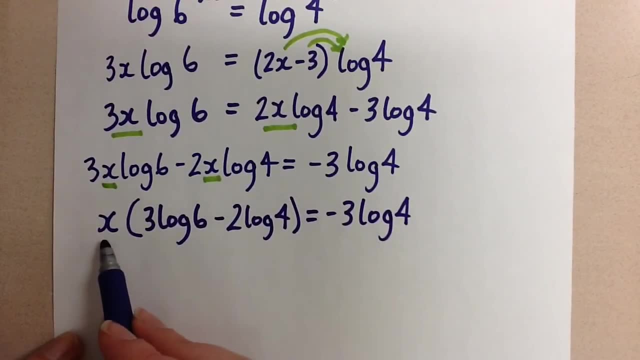 we're left with minus 2, log 4.. And on the right-hand side we still have this. Now we can easily solve for the x, because this is x times a number. This whole thing is just a number here that can be evaluated, So I can divide by that number to get it over to the other side.